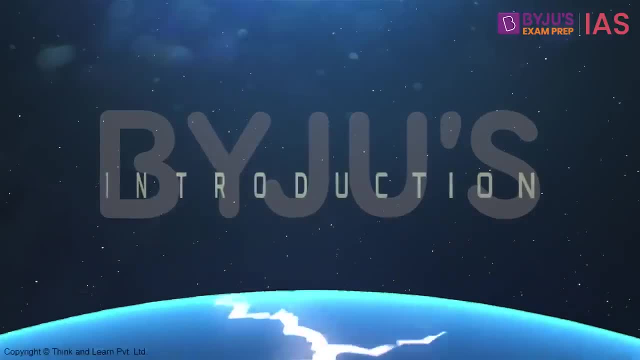 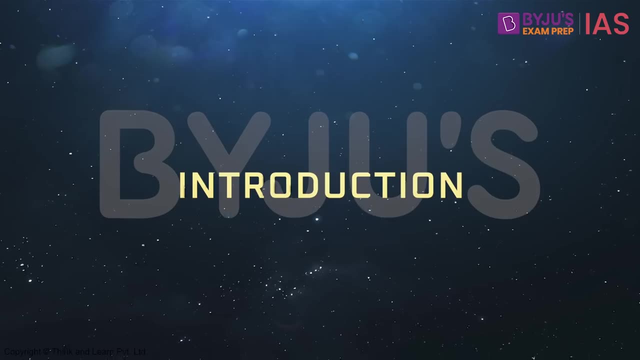 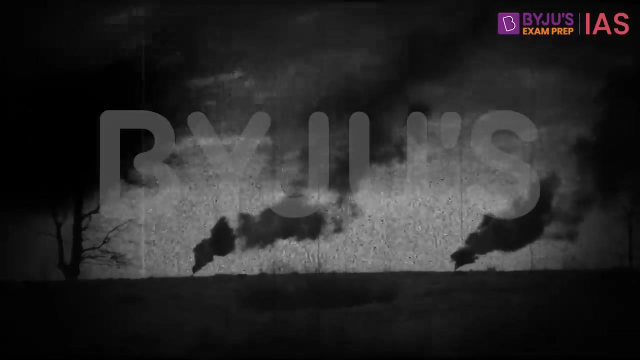 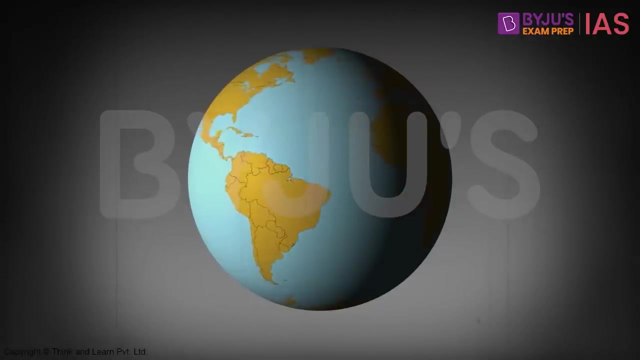 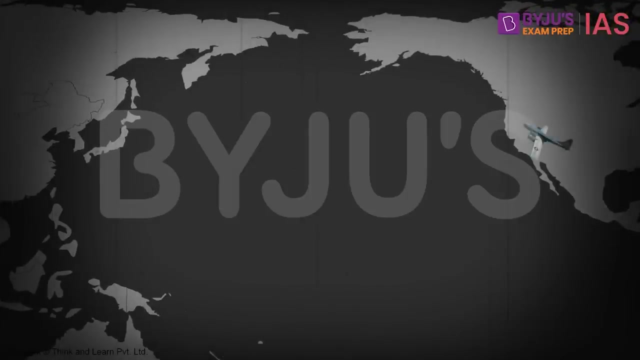 Guns, tanks, planes- nothing was spared, All for the ultimate victory. But among all of this chaos and tragedy, something happened that made our understanding of our own atmosphere much better. It was an incident that happened with American bomber jets that flew from the US to Japan, While the jets were traveling from east to west, that is. 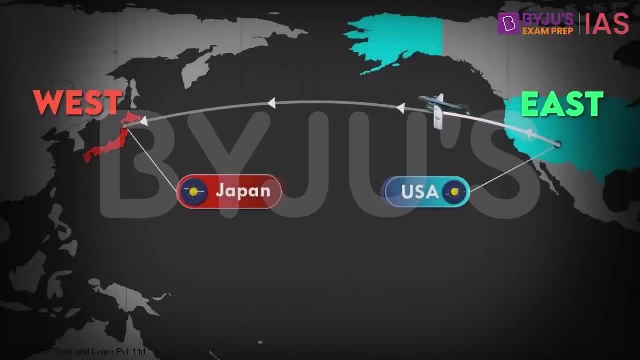 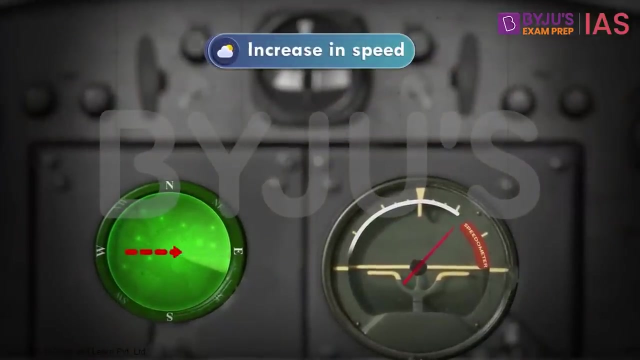 starting from the US and going towards Japan, these jets observed a significant reduction in their speeds. On the other hand, while coming back to the US from Japan, that is, from west to east, they used to witness an increase in their speeds After careful study. 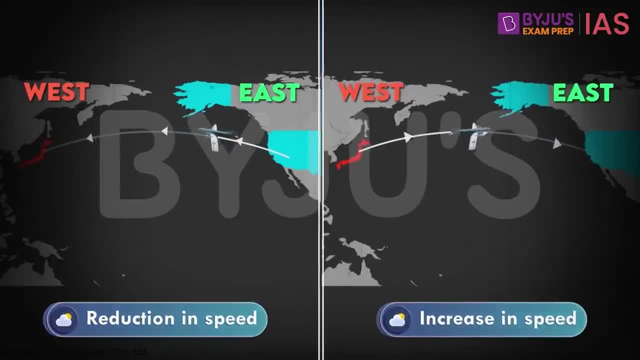 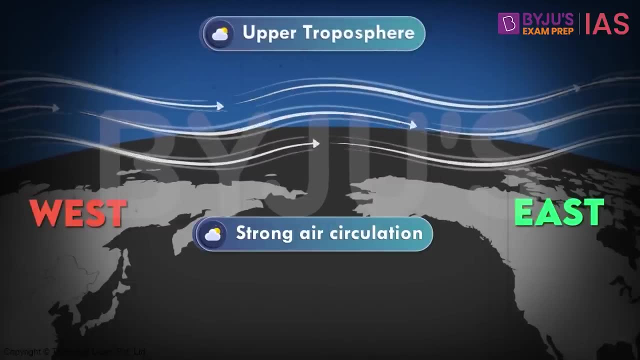 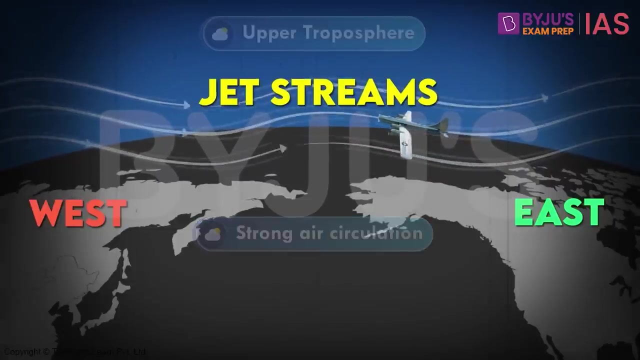 of this phenomenon. It was found that there was a strong air circulation from west to east in the upper portion of troposphere which obstructed the free movement of these jet fighters. this strong air circulation was later named as jet streams. so what are these jet streams? how are they formed? where are they located? 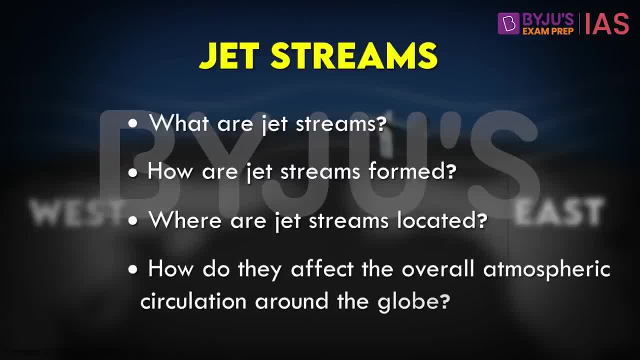 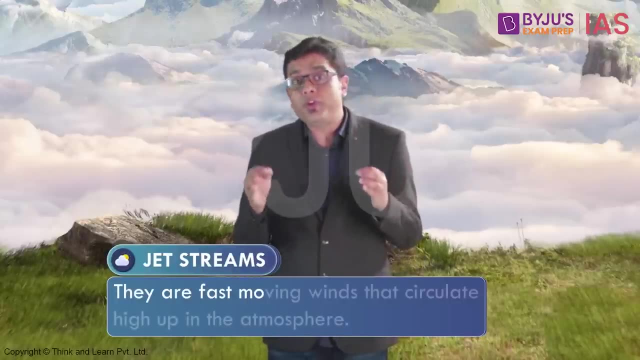 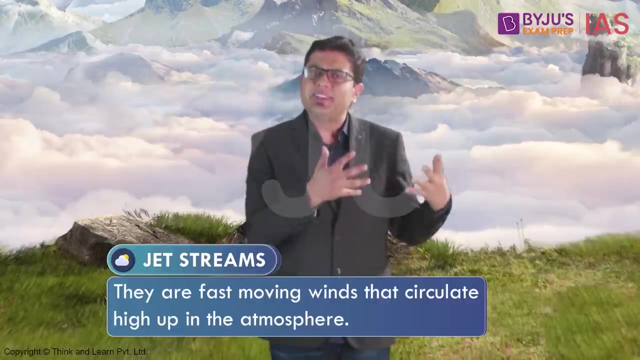 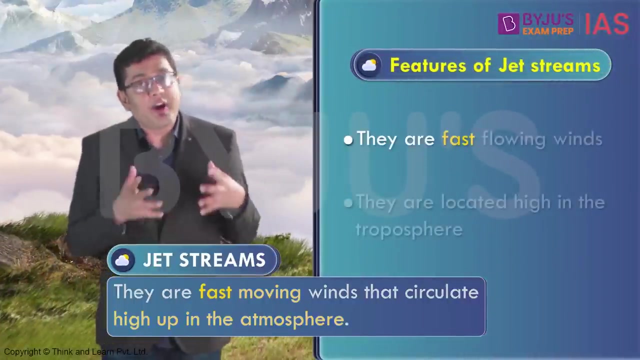 and how do they affect the overall atmospheric circulation around the whole globe? let's start by defining what a jet stream is. so jet streams are fast moving winds that circulate high up in the atmosphere. now, from this definition, we get two pieces of information. one is that these are fast flowing winds, and the other piece of information is that they are located. 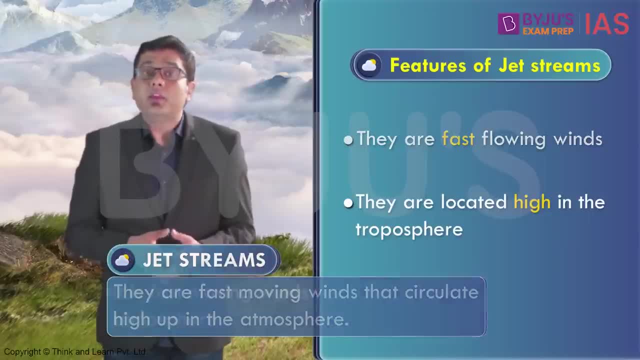 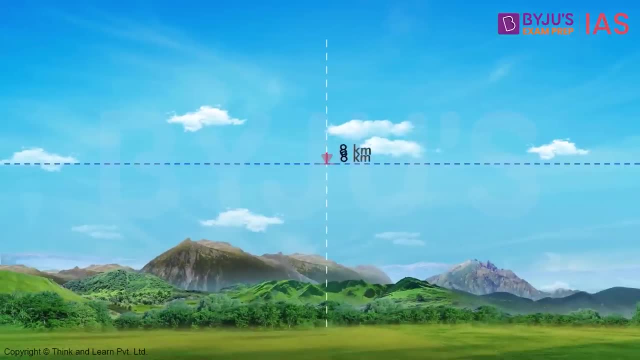 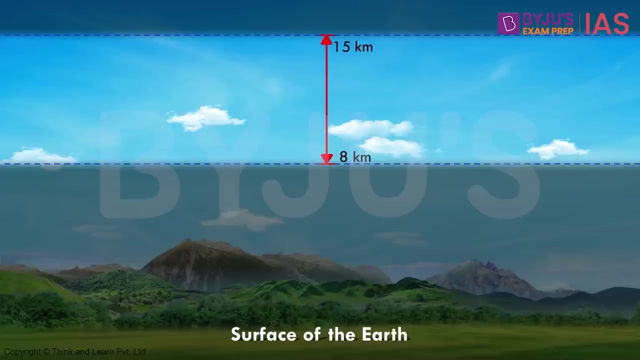 high in the atmosphere. okay, so how high? well, the height ranges somewhere between 8 to 15 kilometers above the surface of the earth. we can say that it is around the region of upper troposphere in itself and, yes, this is almost the same height at which most of the aeroplanes fly. 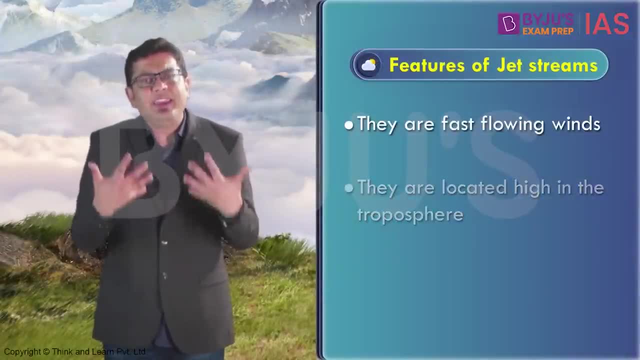 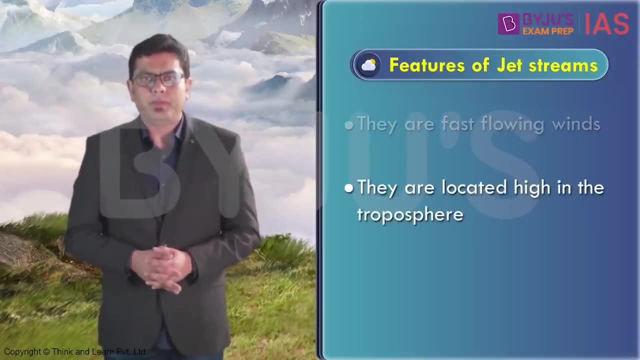 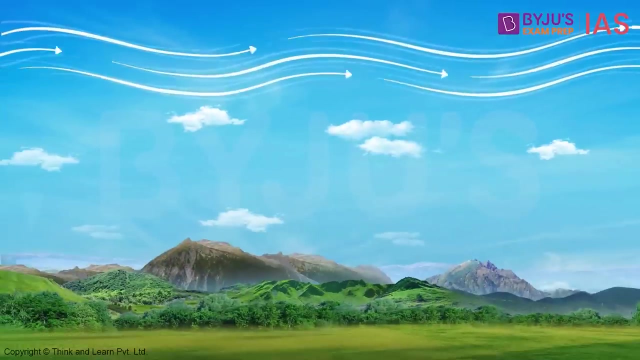 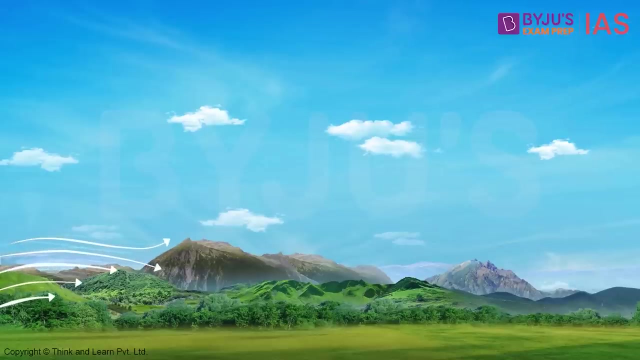 now, the reason for these winds having very high speeds can be explained by their location in the upper troposphere. how is that? well, these winds? they blow at a higher level, the winds that flow close to the surface of the earth. they experience a lot of frictional trap, especially. 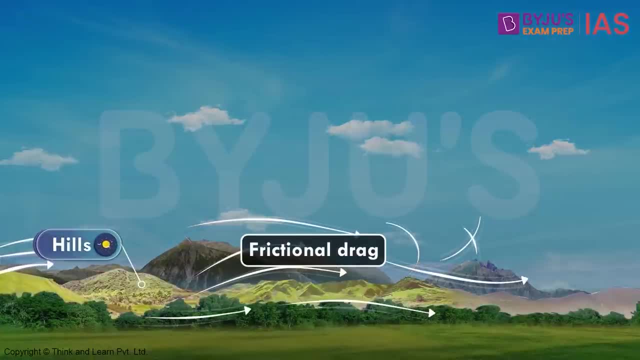 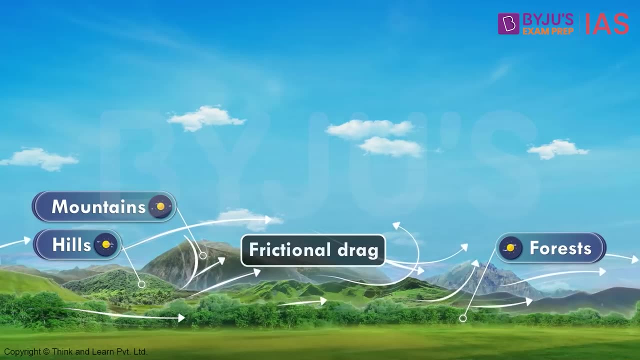 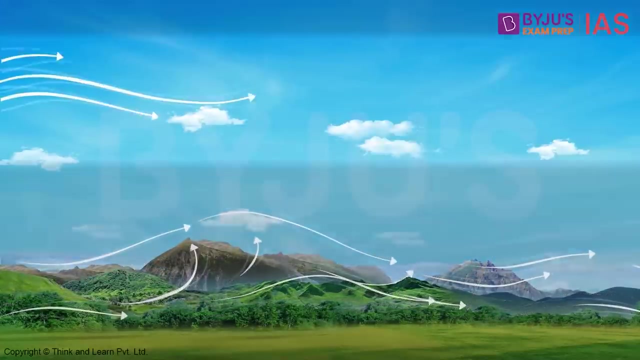 in areas with physical features such as hills, mountains, trees, forests and so on. all these they hamper the wind speed in itself. at the same time, the upper troposphere has relatively low frictional track and hence the wind gets really complicated when it's a naturalightcies or言etry. air flow below aומר. 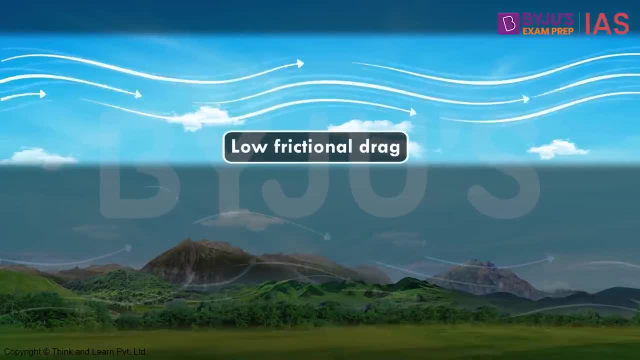 and hence the wind gets functionally heavy when it's the lowest in the atmosphere, being paralyzed. can you Polish this for me, please, Birstenstein, please. that is why we can clear it soon. winds attain very high speeds. Just to give you some numbers: the speed of the jet streams. vary between 129 and 225 kilometers per hour, And in some cases the speeds can reach even up to 443 kilometers per hour. One way to visualize these jet streams is to consider them as rivers. River currents are generally the strongest in the center and decrease in. 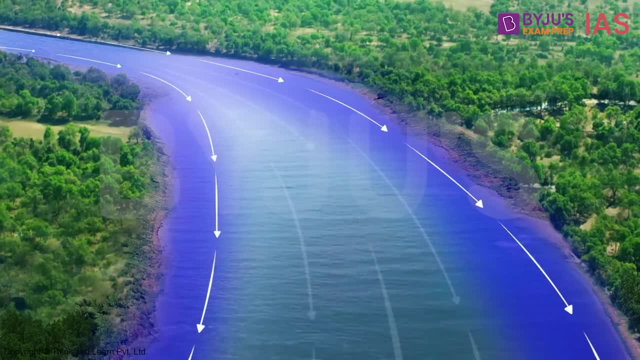 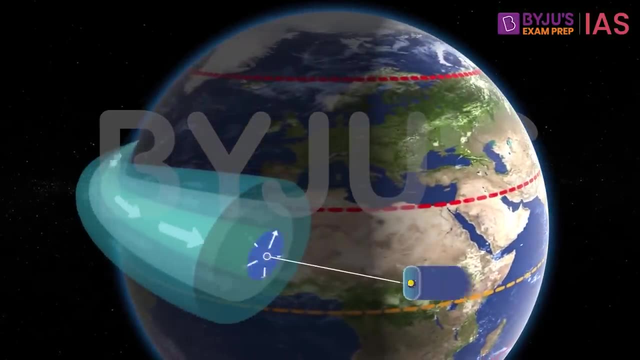 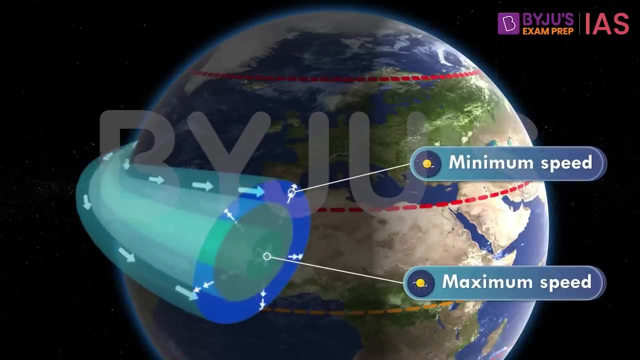 strength as one approaches the riverbanks. This applies to jet streams as well. The speed of a jet stream is maximum at the center and it reduces as we move towards or approach the edges. So we can consider these jet streams as rivers of strength. 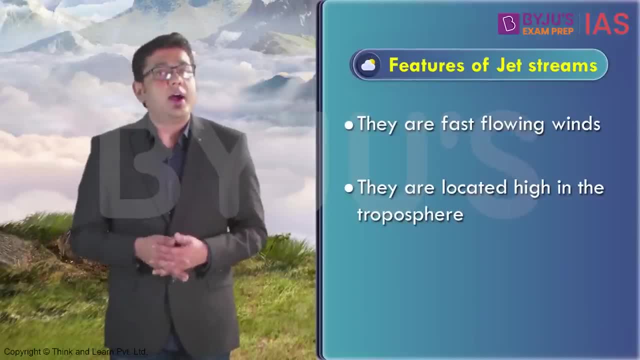 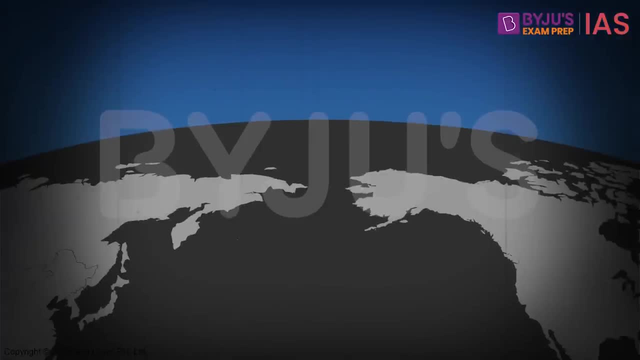 Now we can notice another feature of jet streams from the story we saw earlier. Can you guess it? It is the direction: The planes felt an increase in their speeds when traveling from west to east. Thus the jet streams were aiding the planes. Thus it is clear from 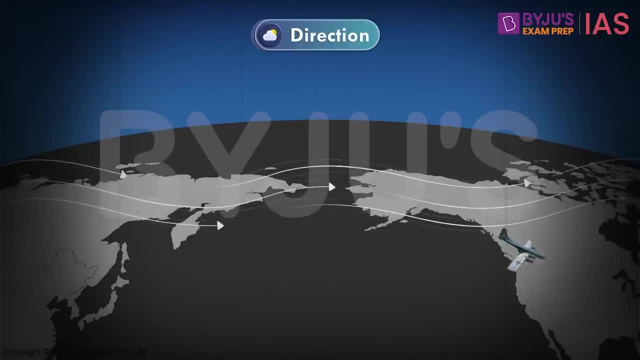 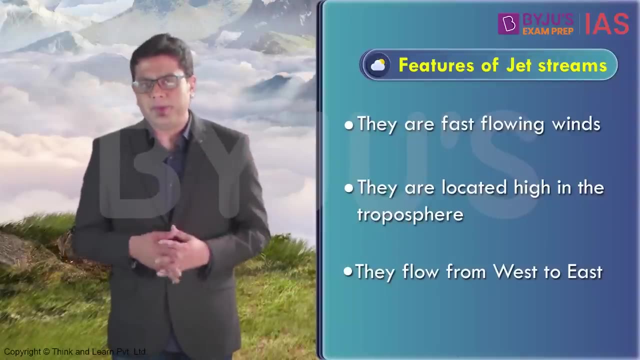 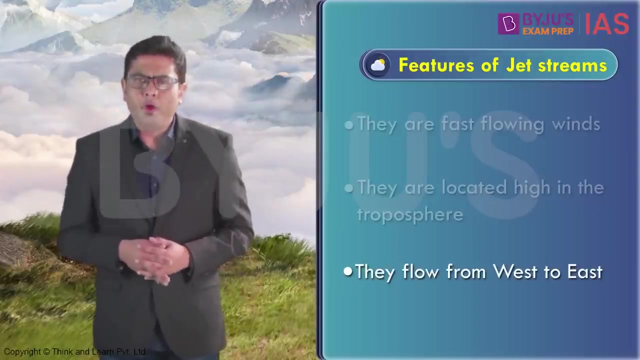 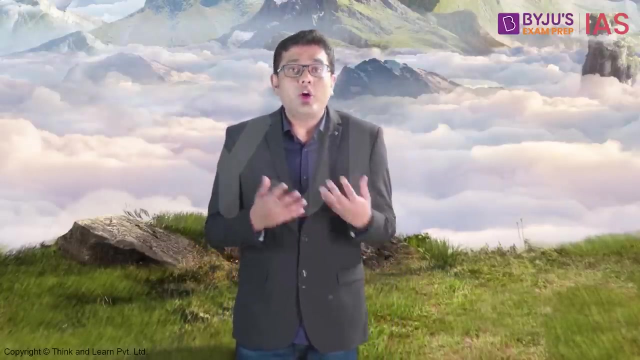 the above example that the direction of the jet streams is from west to east. So now we know three things about jet streams. They are fast, They flow in the upper troposphere And they flow from west to east. Are you curious to know if all jet streams are the same or if there are different types? 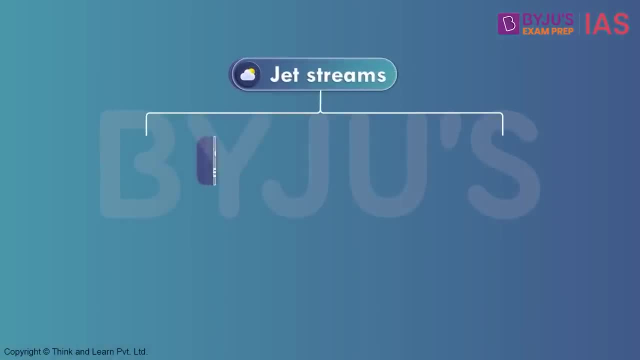 Well, there are two different types of jet streams: One is the top and the other is the: the permanent jet streams and the temporary jet streams. Permanent jet streams are those which exist throughout the year, while temporary jet streams are formed in a specific location for a limited period of time, Since they are 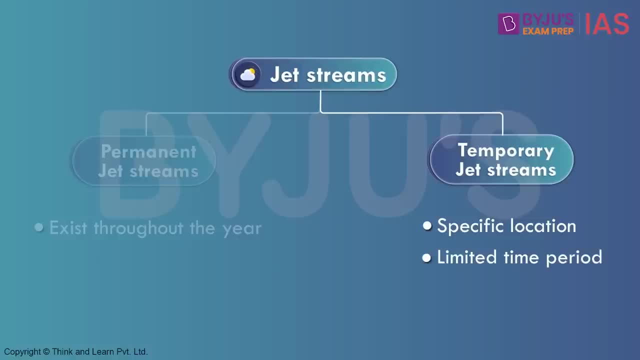 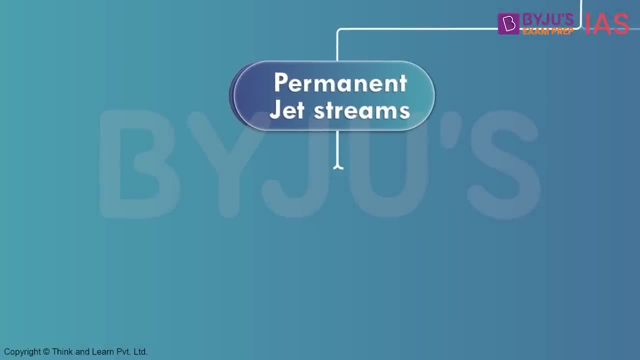 not present throughout the year, they are called as temporary jet streams. Now coming to the permanent jet streams, there are two major examples in this category: The subtropical westerly jet streams and polar front jet streams. While under temporary jet streams we have the examples of the tropical 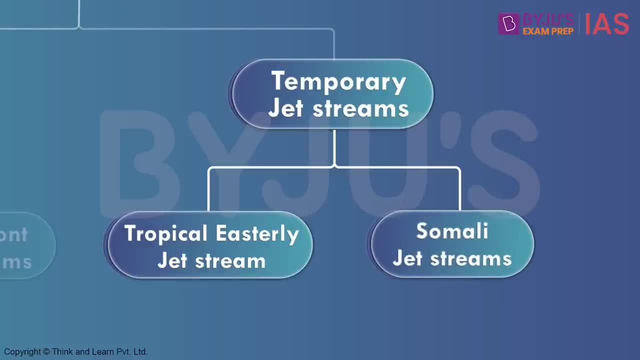 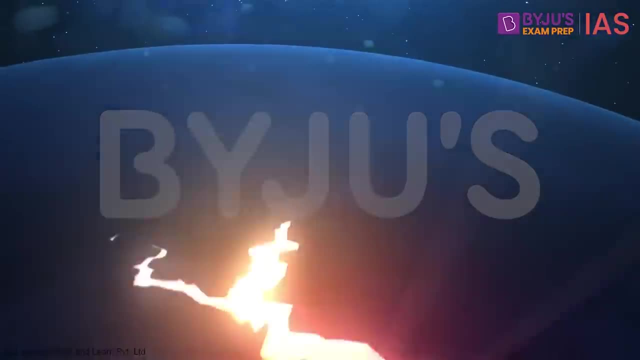 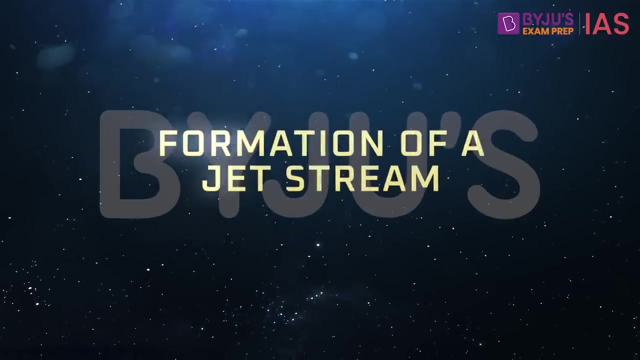 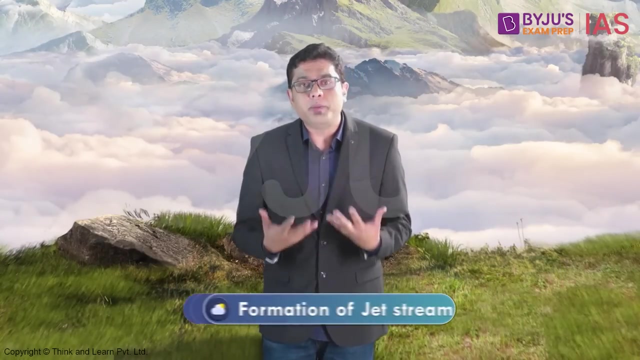 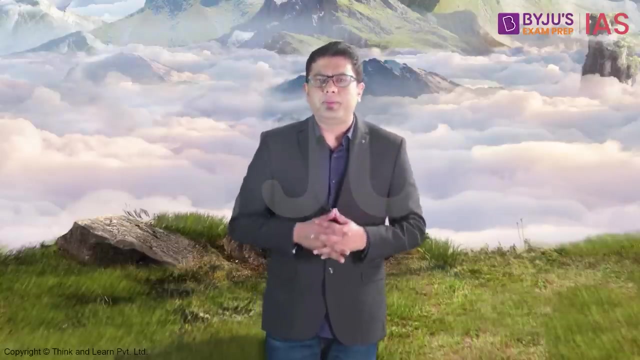 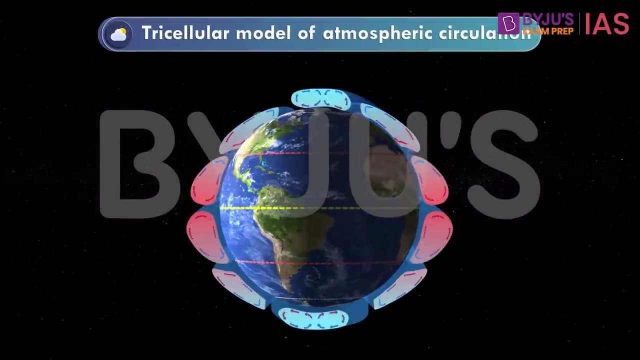 easterly jet stream and the Somali jet stream. Okay, so that was all about the different types of jet streams. Now let's discuss the formation of jet streams. Well, before we dive into that part, there are a few concepts that we need to revisit. First, we will look into the concept of the tri-cellular model of 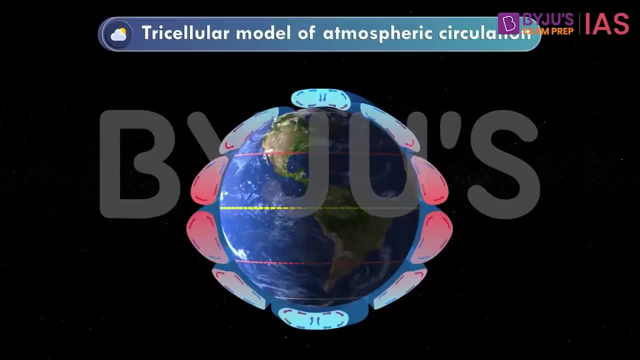 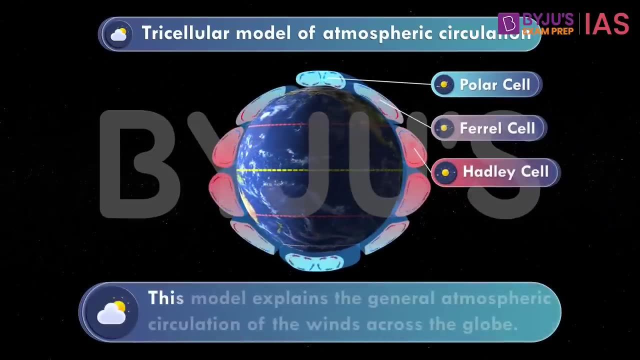 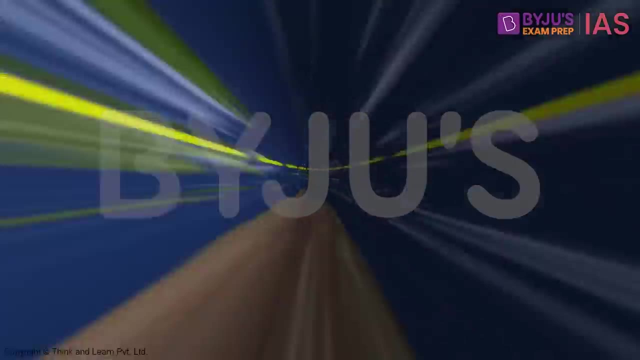 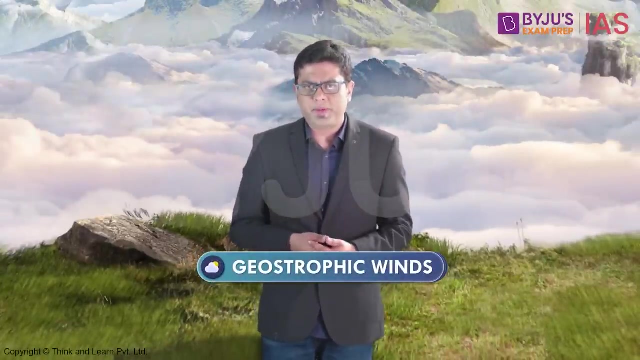 atmospheric circulation. Do you remember the, the Hadley cell, the Ferrel cell and the Polar cell? This model explains the general atmospheric circulation of the winds across the globe. The second concept we need to revise is the concept of geostrophic winds, which result 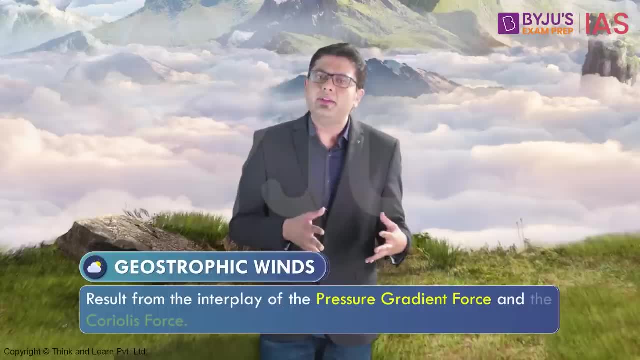 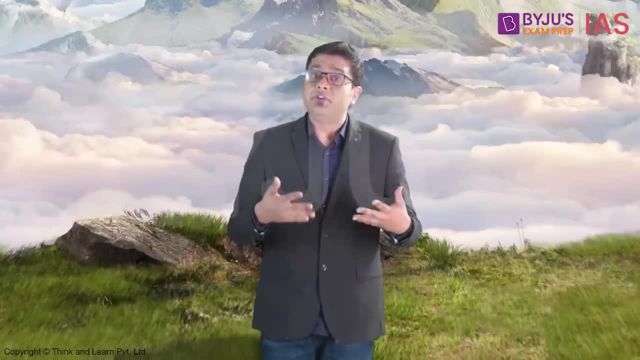 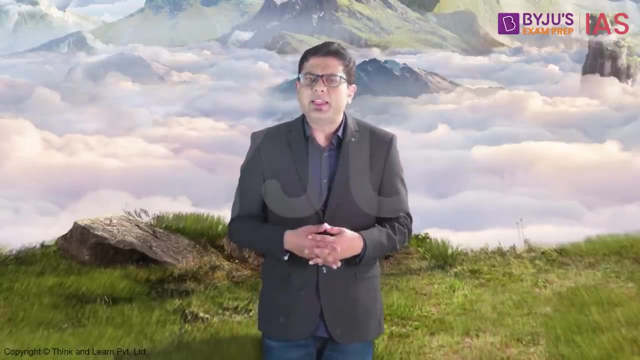 from the interplay of pressure gradient force and the Coriolis force. Now let us understand this with an example. As we know, wind moves when there is a pressure gradient. Let us suppose that these isobars represent different values of pressure present in any area. As you can see, down south we have a high pressure of around 5 bar, and as we move north it decreases to 4, 3,, 4 bar, 3, 2 and finally 1 bar. Now, because of this pressure difference, a pressure gradient force develops from high. 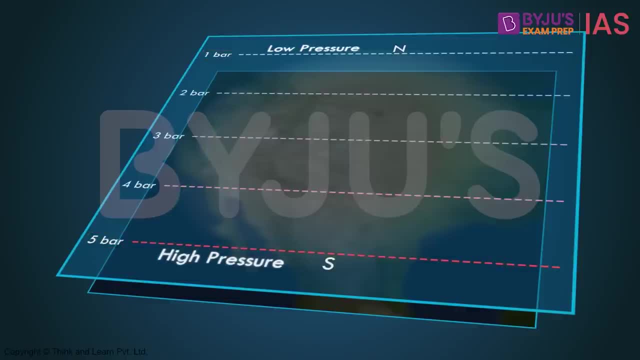 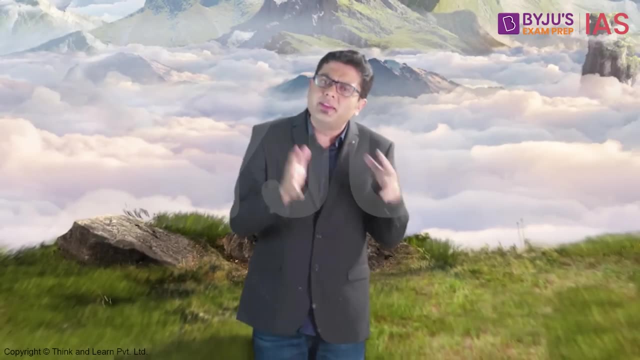 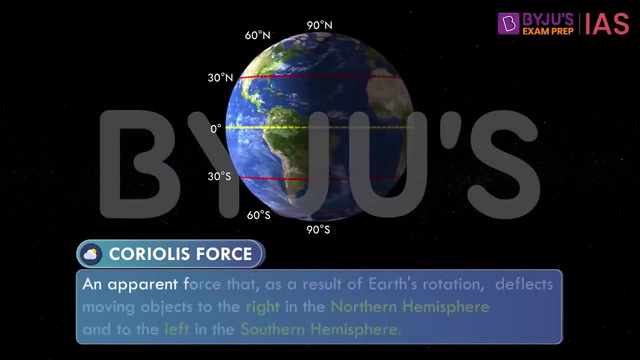 pressure to low pressure, and thus the wind starts moving from south to north. Now let us bring in another factor in the system, the Coriolis force. We know it is an apparent force. It is the result of Earth's rotation, which deflects moving objects to the right in northern 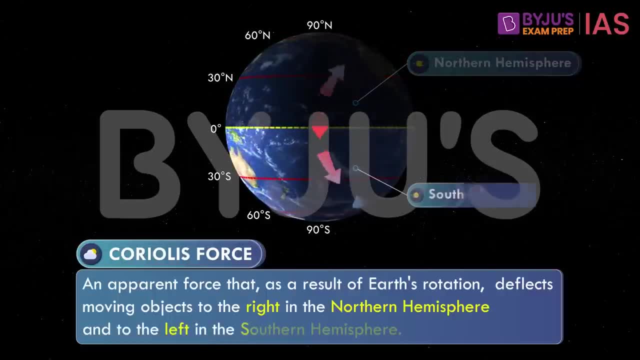 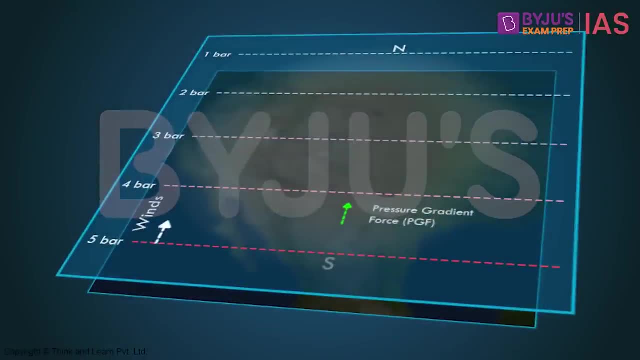 hemisphere and to the left in the southern hemisphere. Let us assume our system is in northern hemisphere, So the Coriolis force will turn the winds towards its right. As the wind speed increases, the effect of Coriolis force increases as well. 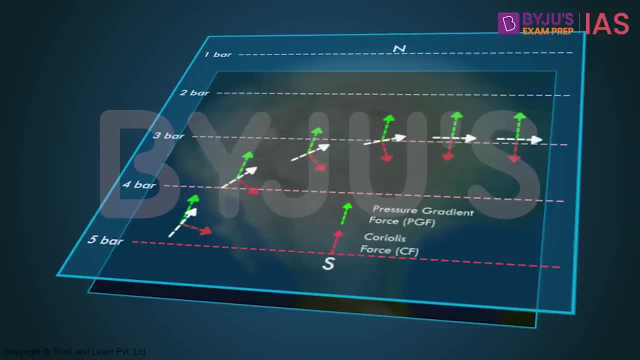 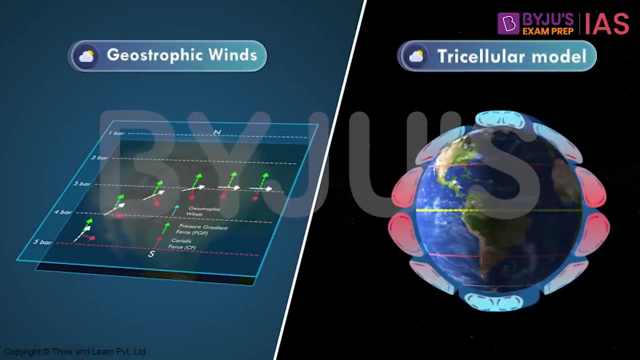 Then comes a point when the pressure gradient force gets balanced by Coriolis force and the resultant direction of the winds become almost parallel to the isobars. Now, with the help of these two concepts, we can understand the origin of jet streams. 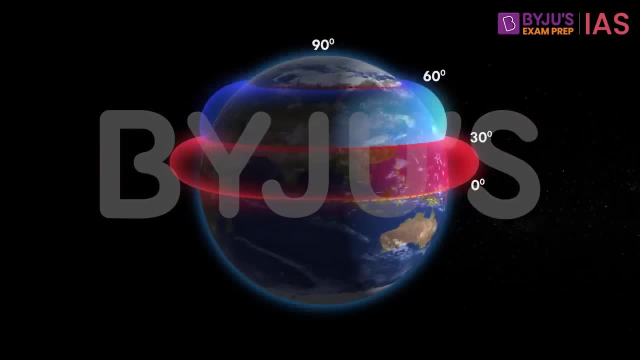 We can understand the origin of jet streams. We can understand the origin of jet streams. streams form when warm air mass meets cold air mass. in the upper troposphere, We know, the air above tropical region is warm, while the air above temperate region is relatively cold. Now imagine two air columns in these two different. 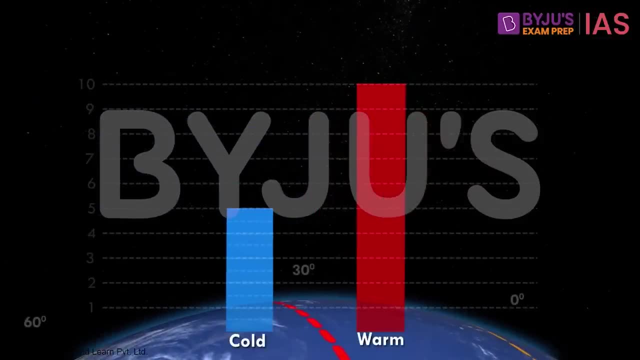 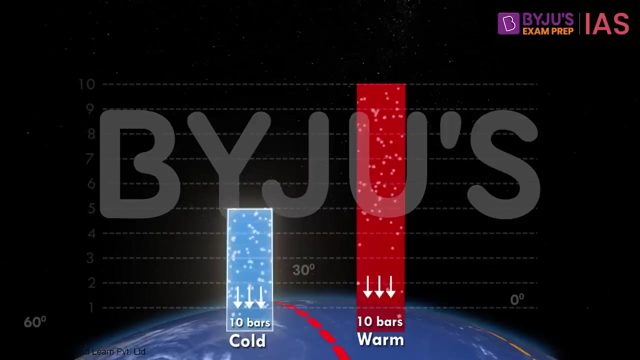 regions. These two columns of air apply the same pressure on the surface of the earth. Let us say hypothetically it's around 10 bars each. Now we know that cold air is comparatively denser. Thus a smaller column of cold air can apply the 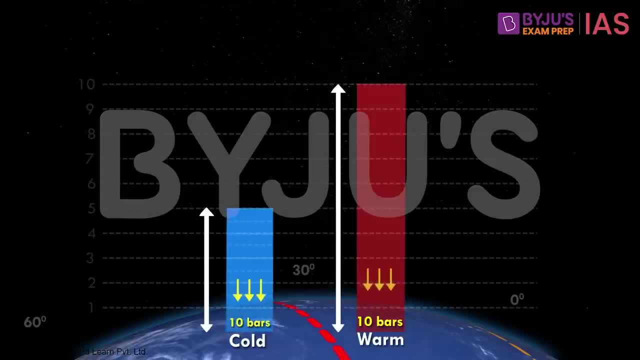 same pressure as a relatively larger column of warm air. Let us assume the height of the warm air column is around 10 units and the height of the cold air column is somewhere around 50. 5 units. Now the fall of pressure in the cold air column will be comparatively 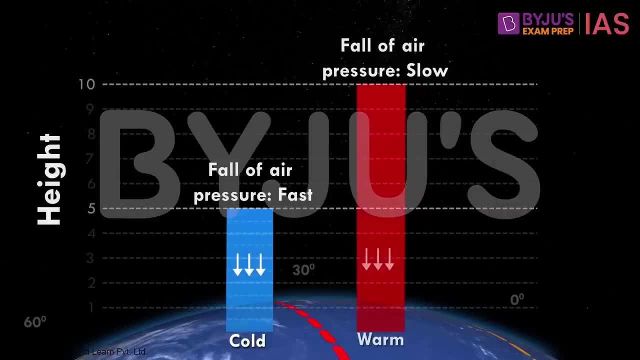 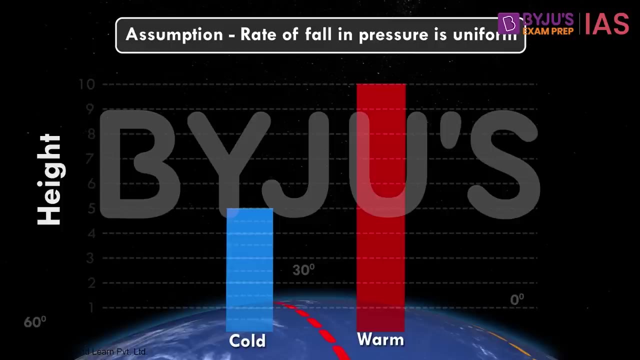 faster when compared to the warm air column. Are you confused? Okay, let us try to understand it in this way. Let us assume the rate of fall in the pressure is uniform in both these cases. So for a warm column of air, the rate of fall in 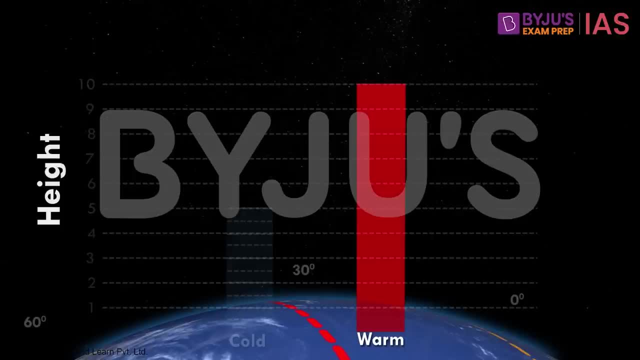 the pressure with respect to height will be somewhat like this, And for cold air column it will be somewhat like this. Here you can see that warm air has a generous 10 units of height to achieve a fall of 10 bars of pressure, While the 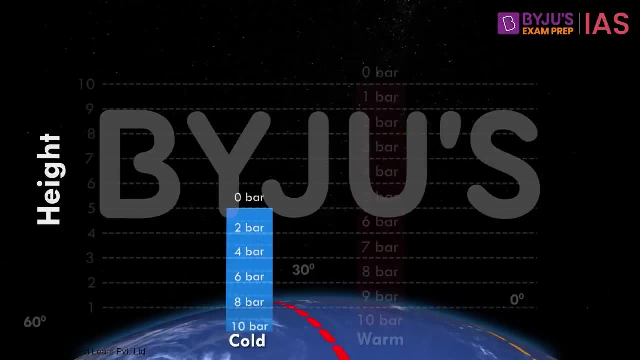 cold air column has to achieve the same fall within a mere 5 units of height, And thus the fall in this case shall be considerably faster. Now let us take a specific height, Say 3 units from the surface of the earth itself. Note the pressure values for both these columns. 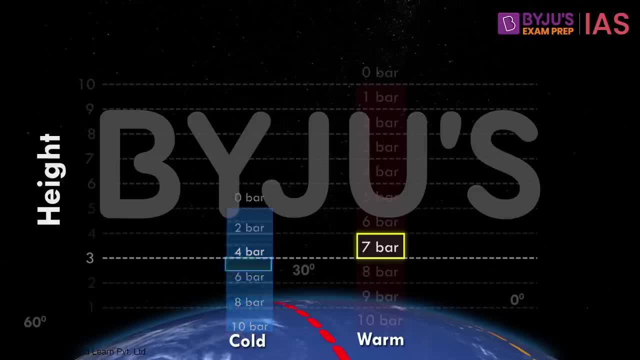 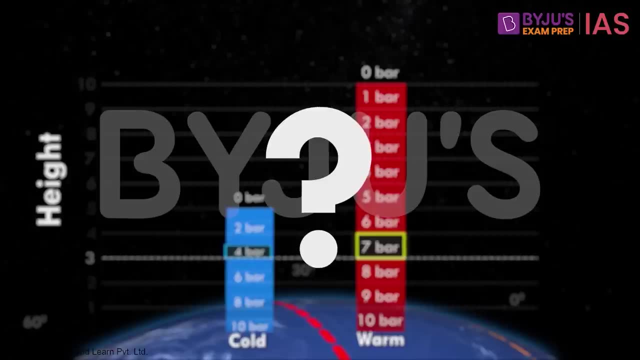 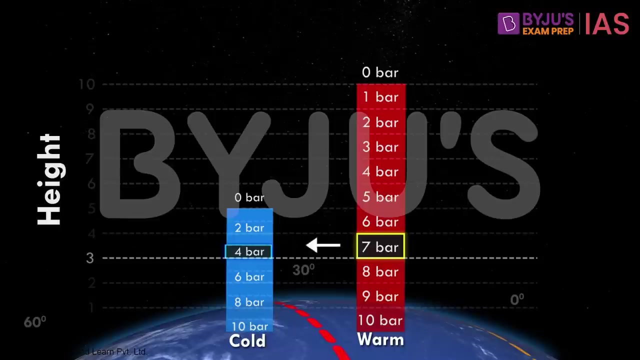 7 bar for warm and 4 bar for cold. So what will be the pressure gradient And in which direction will the wind actually flow? Well, it will flow from the warm air column towards the cold air column. Something similar happens in the upper reaches of troposphere as well. 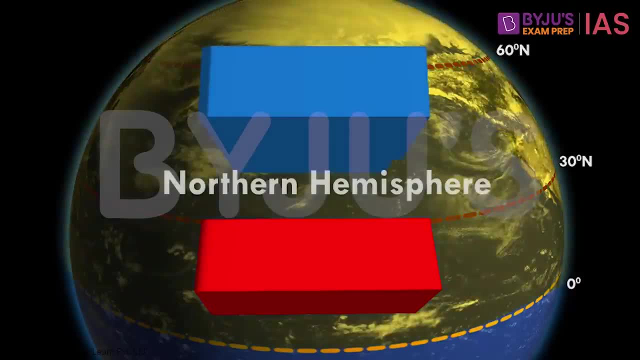 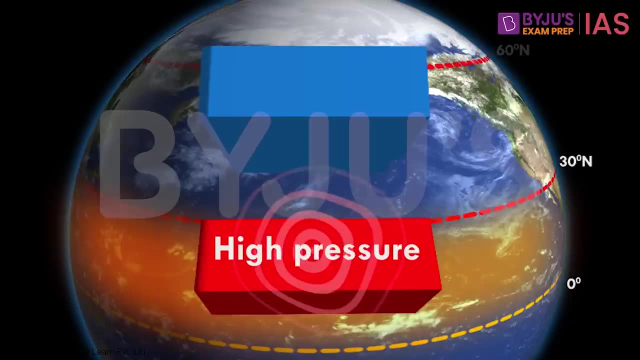 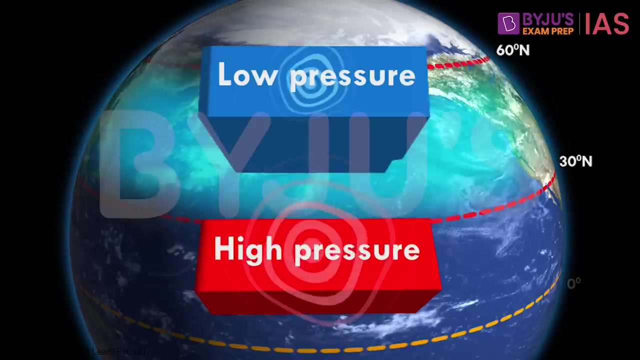 If we assume we are in the northern hemisphere, then a high pressure will develop in the warm air mass of the tropical regions and simultaneously a low pressure will develop in the cold air mass of the temperate regions. Thus the flow of the wind shall be from south to north. 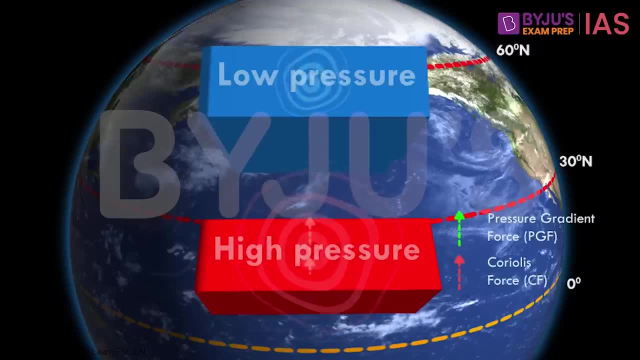 Now, as the air moves, the Coriolis force continues to act on it and it deflects the wind towards the right. As the wind speed continues to increase, the effect of Coriolis force increases and there comes a point when the pressure gradient force. 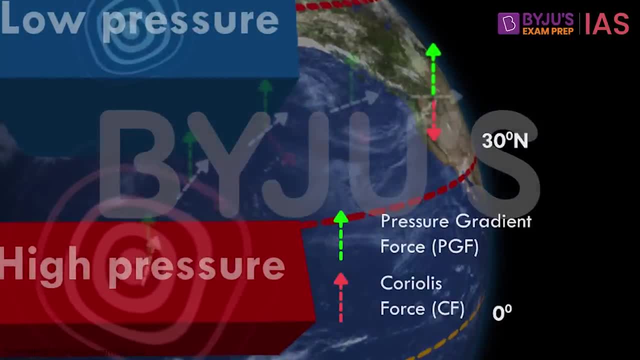 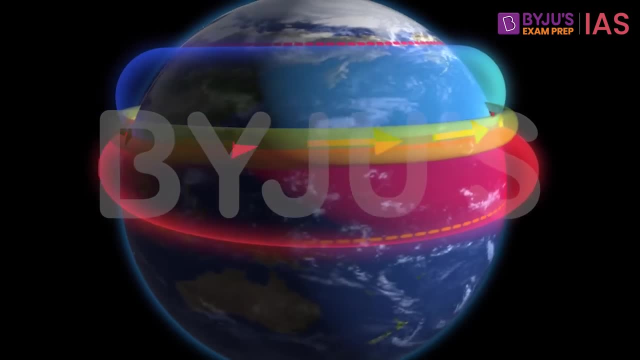 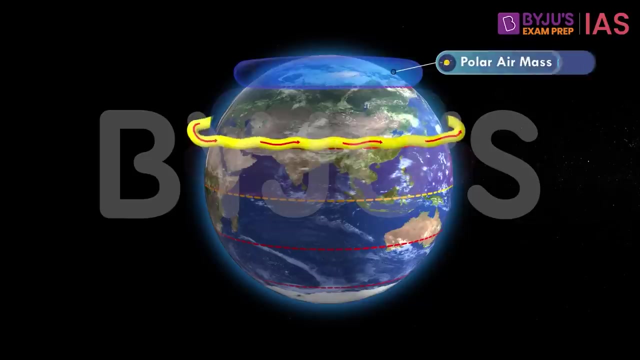 gets balanced by the Coriolis force, and the resultant direction is from west to east. Now something similar happens in higher latitudes as well. When the cold air mass from polar region interacts with relatively warm air mass from the temperate regions, we get the following effect: 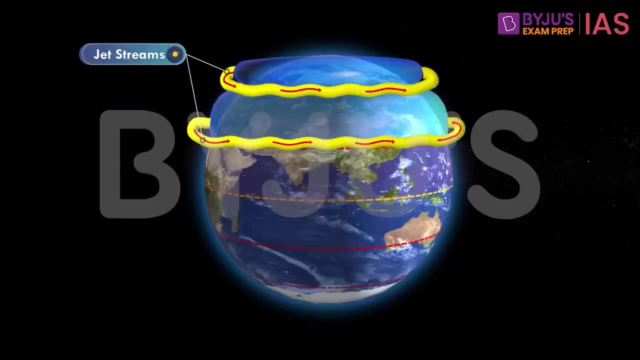 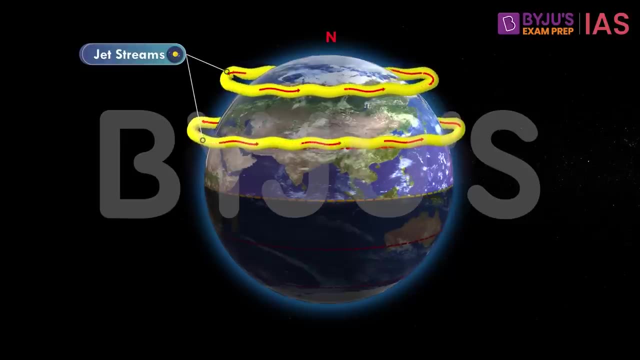 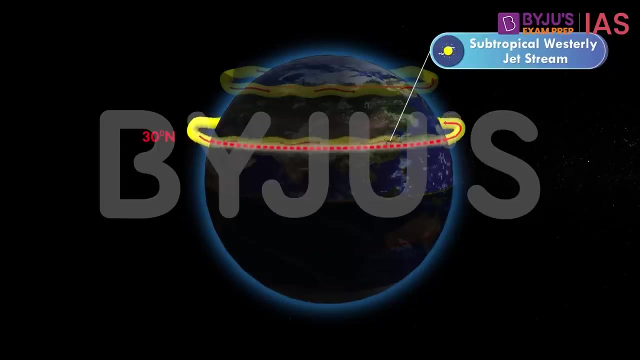 We get a jet stream again. Thus, we saw two jet streams form in the northern hemisphere, While the first one is called the subtropical westerly jet stream. it is formed around 30 degree latitude at the boundary of interaction between the Hadley and the Ferrel cells. 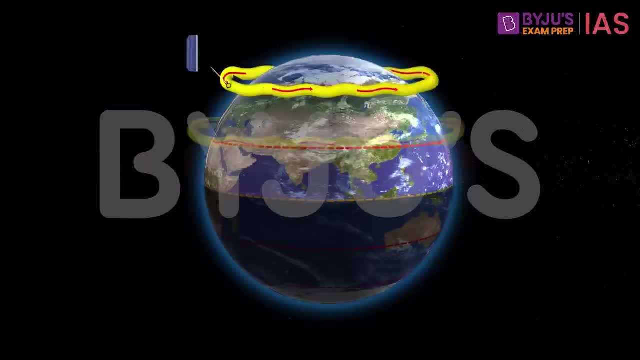 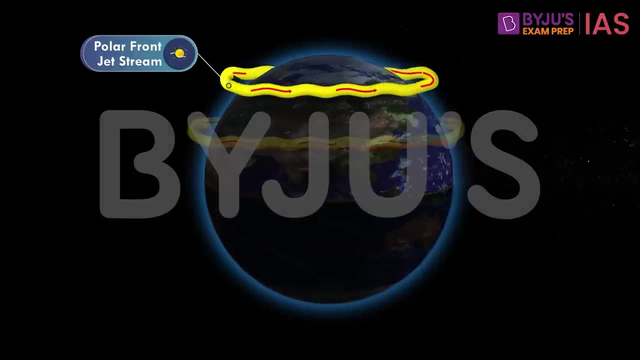 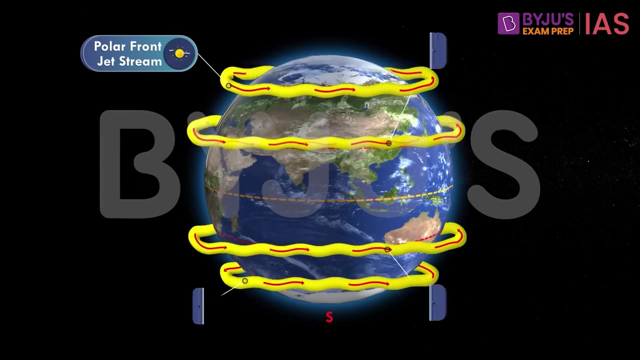 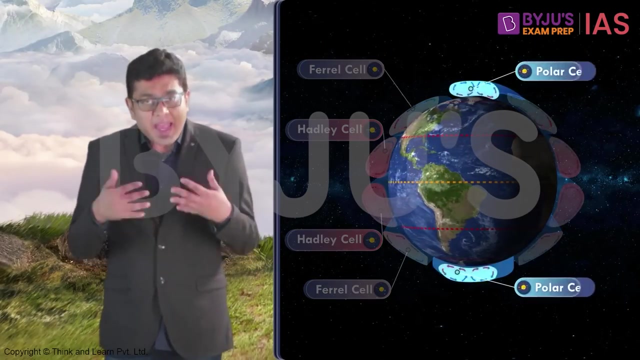 The other one is called as the polar front jet stream. It is formed somewhere around 60 degree latitude at the boundary of the Ferrel and the polar cells. Now in the southern hemisphere we can see two similar jet streams: The Hadley Ferrel polar cells and the pressure belts are permanent. 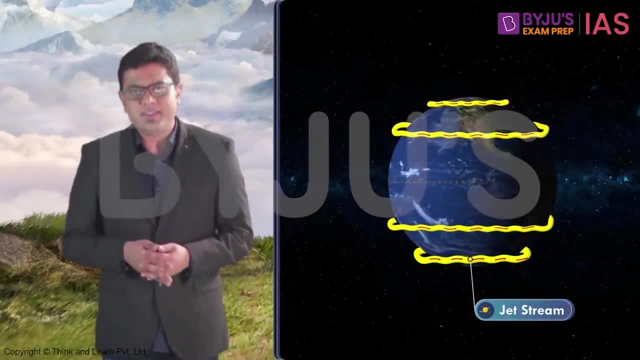 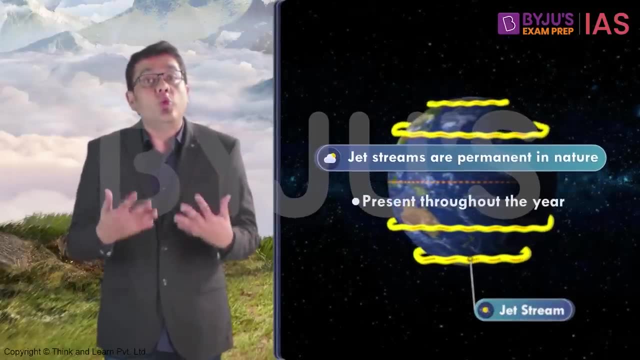 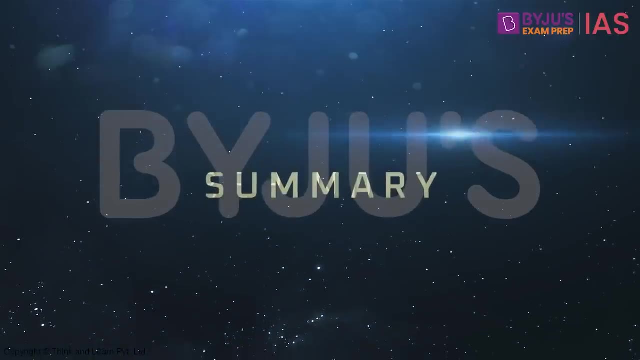 Since the jet streams are formed due to interaction of these cells, they are permanent as well. In other words, the jet streams are present throughout the year. As the atrocities occur in the cold air, the jet streams are still present throughout the year. 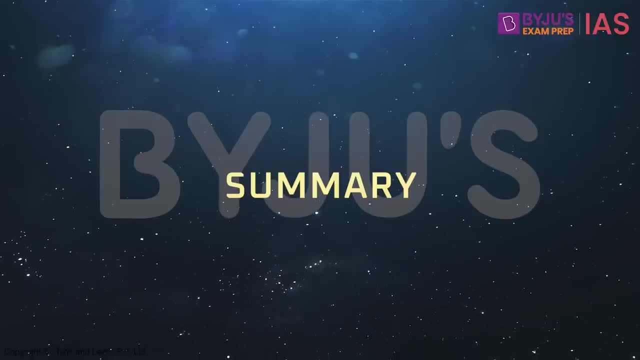 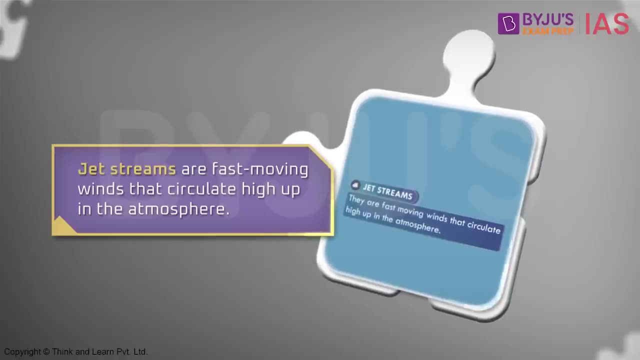 The jet streams from the orbit and the distance of the setback remain permanent during the entire time. The jet stream is moving, increasing its capacity to reach the polar�ar. The jet stream is moving, increasing its capacity to reach the polar�ar.